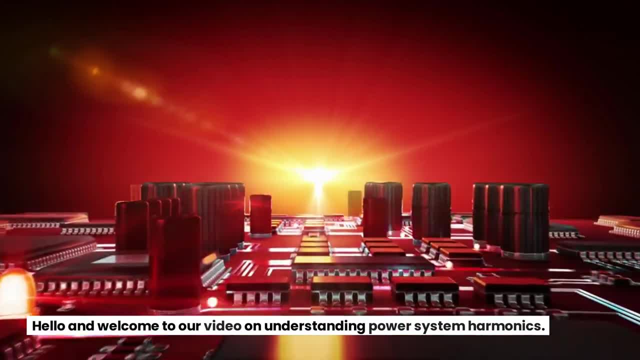 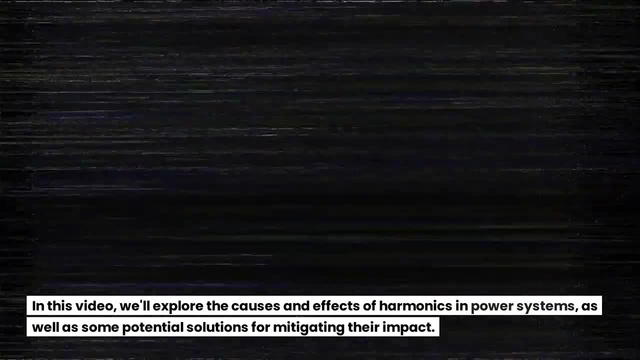 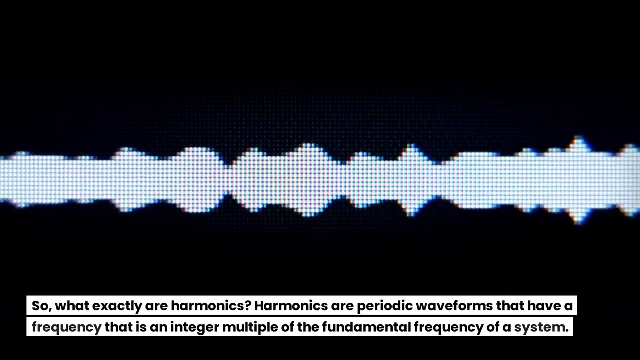 Hello and welcome to our video on understanding power system harmonics. In this video, we'll explore the causes and effects of harmonics in power systems, as well as some potential solutions for mitigating their impact. So what exactly are harmonics? Harmonics are periodic waveforms that have a frequency that 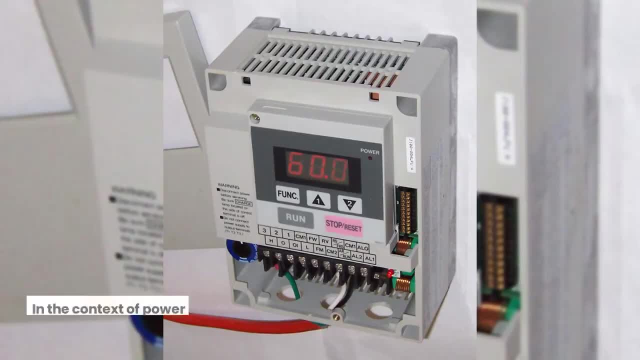 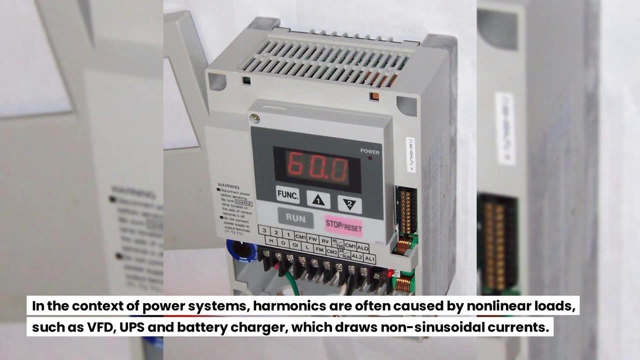 is an integer multiple of the fundamental frequency of a system. In the context of power systems, harmonics are often caused by nonlinear loads, such as VFD, UPS and battery charger, which draws non-sinusoidal currents. This can cause the voltage and current in the 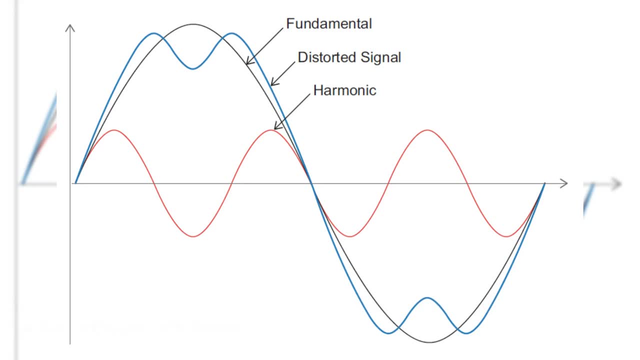 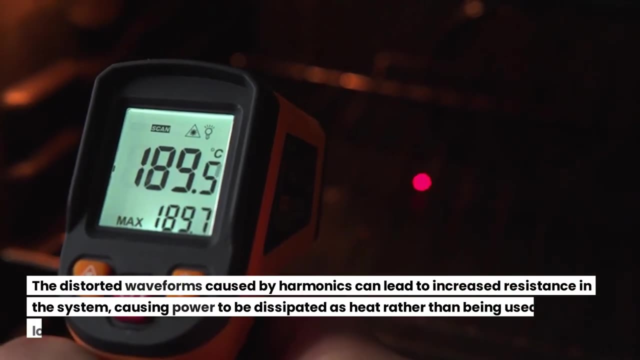 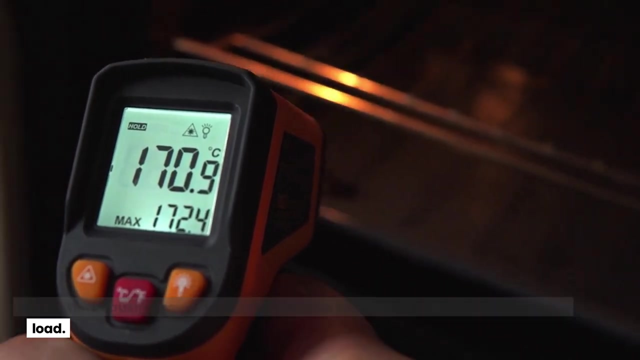 system to become distorted, which can lead to a number of problems. One of the main effects of harmonics in power systems is increased power loss and heat generation. The distorted waveforms caused by harmonics can lead to increased resistance in the system, causing power to be dissipated as heat rather than being used by the load. This can lead to 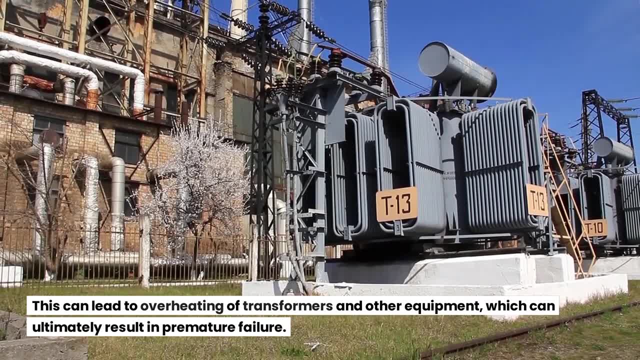 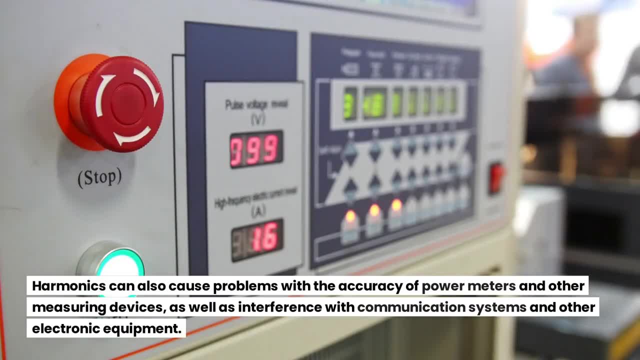 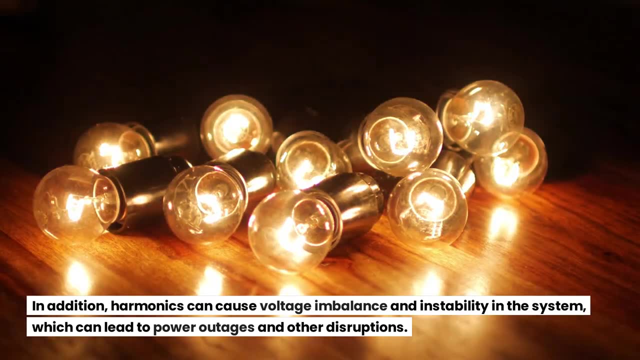 overheating of transformers and other equipment, which can ultimately result in premature failure. Harmonics can also cause problems with the accuracy of power meters and other measuring devices, as well as interference with communication systems and other electronic equipment. In addition, harmonics can cause voltage imbalance and instability in the system. 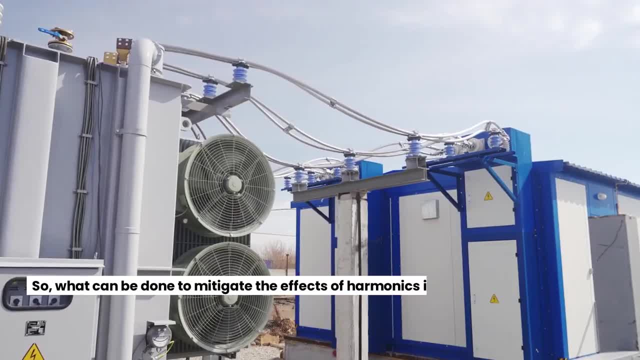 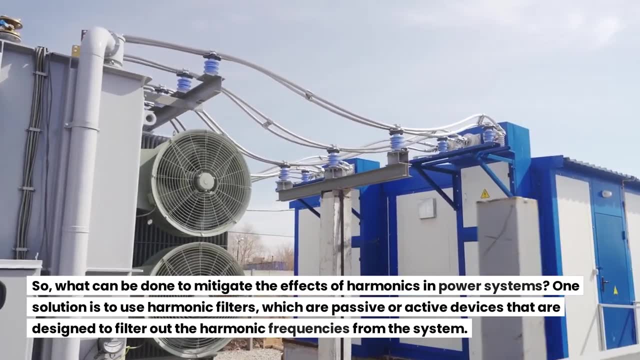 which can lead to power outages and other disruptions. So what can be done to mitigate the effects of harmonics in power systems? One solution is to use harmonic filters, which are passive or active devices that are designed to filter out the harmonic frequencies from the system. 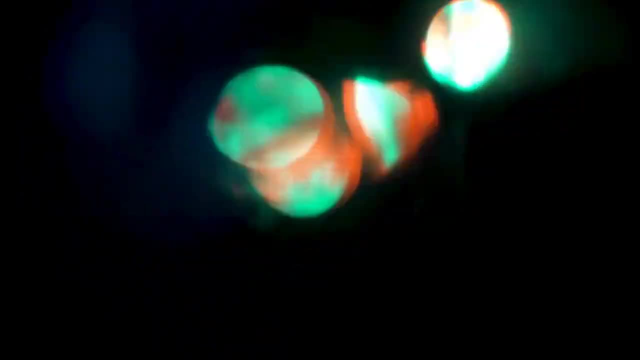 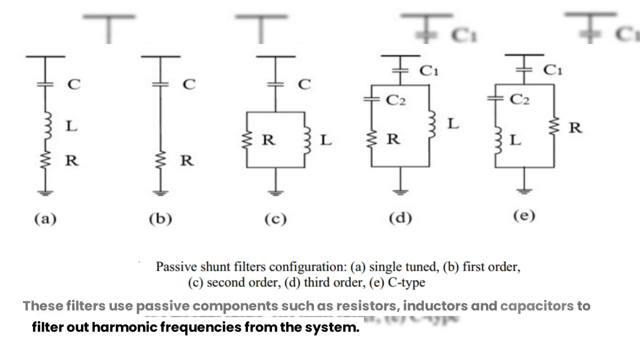 Let's discuss them one by one. Passive filters: These filters use passive components such as resistors, inductors and capacitors to filter out harmonic frequencies from the system. Passive filters are simple and cost-effective, but they have somewhat limited effectiveness as 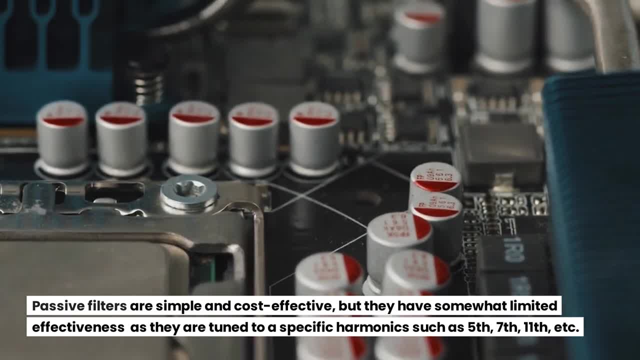 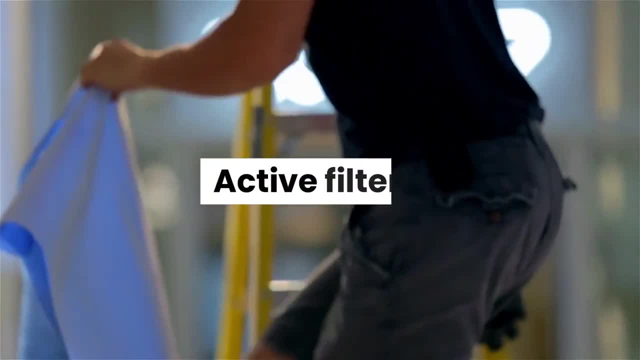 they are tuned to a specific harmonics, such as 5th, 7th, 11th, etc. Real-time compensation is not possible with passive filters- Active filters. Active filters can automatically reduce current harmonics in a network across a broad frequency spectrum. 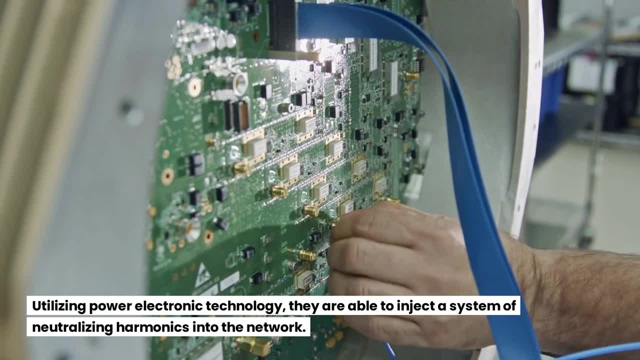 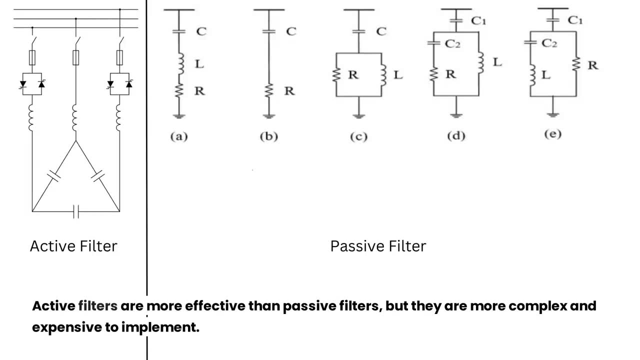 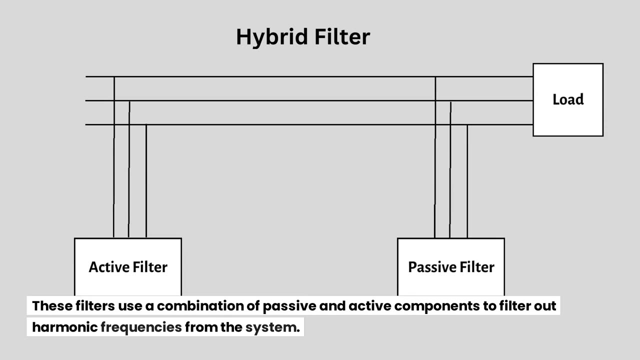 Utilizing power electronic technology, they are able to inject a system of neutralizing harmonics into the network. Active filters are more effective than passive filters, but they are more complex and expensive to implement. Hybrid filters: These filters use a combination of passive and active components to filter out.